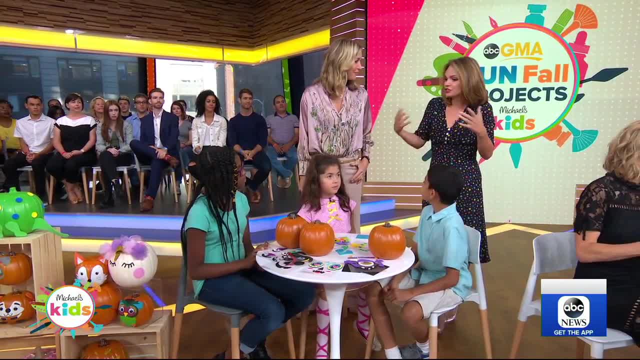 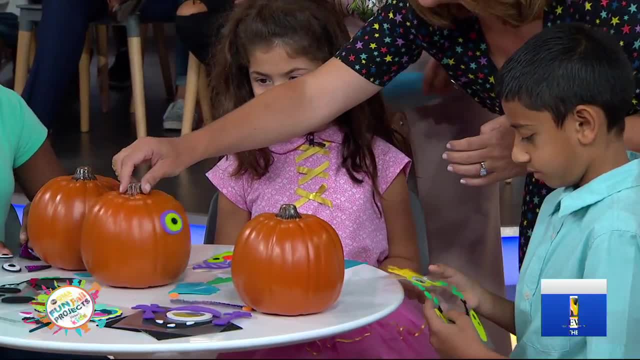 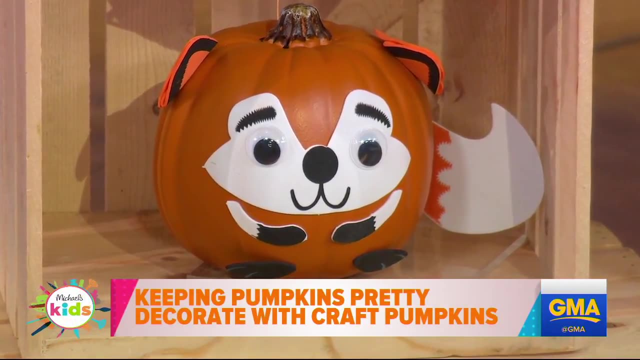 Here we have all of our friends. We are sticking on foam stickers. You can make eyes. I love this. I love it. These are craft pumpkins. It's not as messy. That's why I love a craft pumpkin. As you said, we can go ahead and get in here. 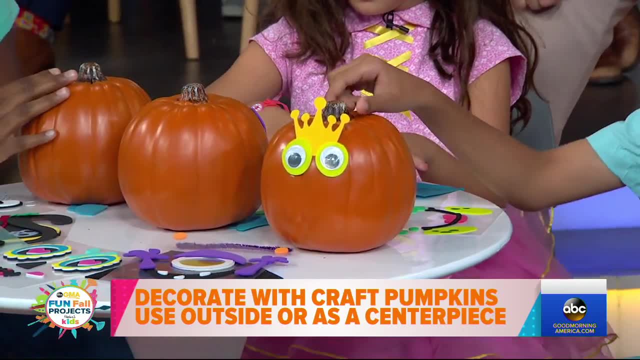 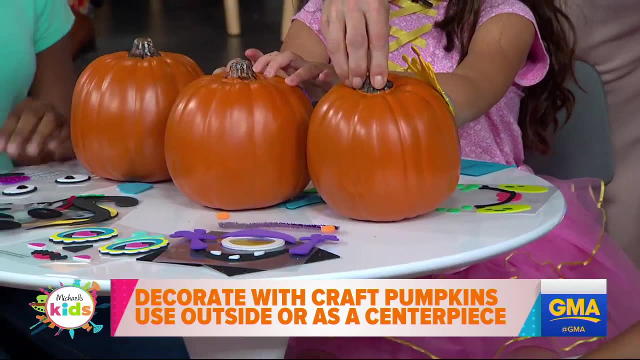 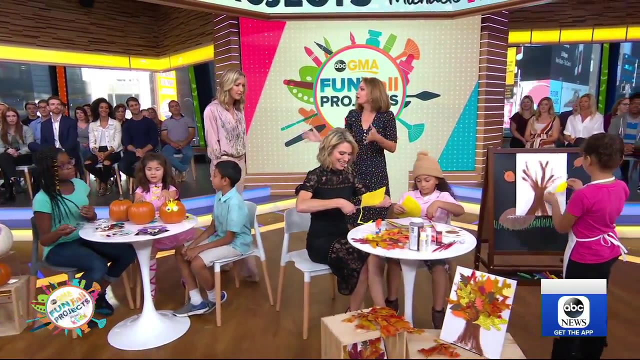 No two are alike. This is about making it fun and making it easy and doing an activity with your kids screen free. That is our favorite part. That's the pumpkin prince. We did a good job. Amy has been working hard with these guys. 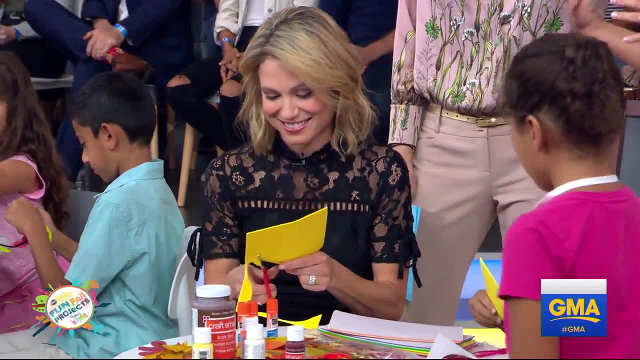 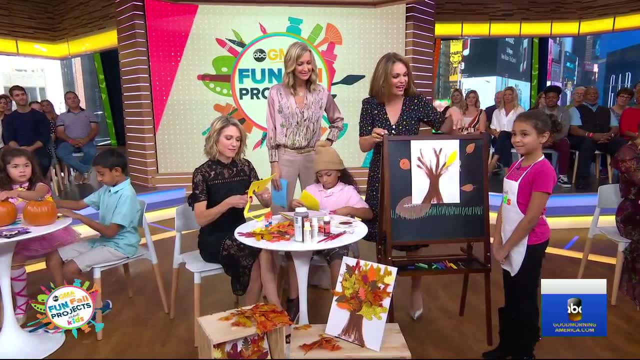 I'm so impressed. This is all about bringing the outdoors in for fall. You can buy this easel on michaelskidscom. Here we have our friend. She's doing a tree. She's sticking all these fall stickers, foam stickers, on to. 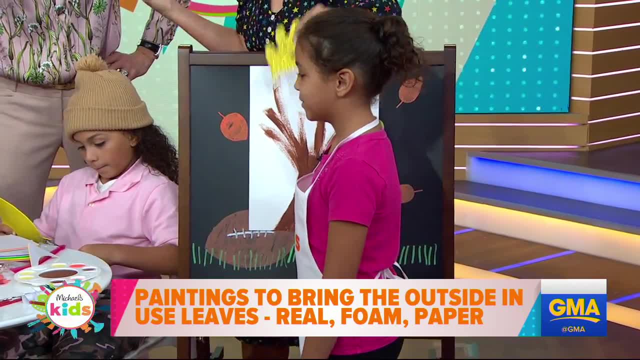 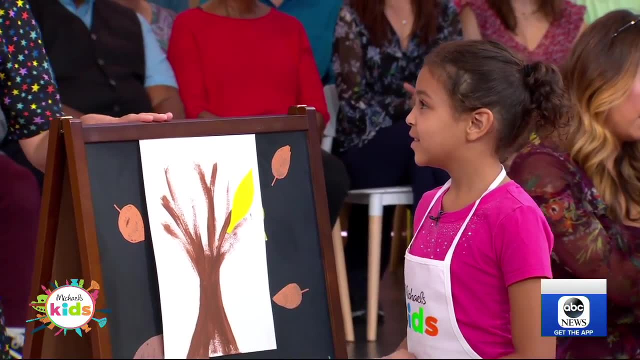 really jazz it up Again, bringing in the fall season. What do you think of this project? I think it's nice and I like it. It's nice, More fun than video games, right? Right, It's all about making it easy. 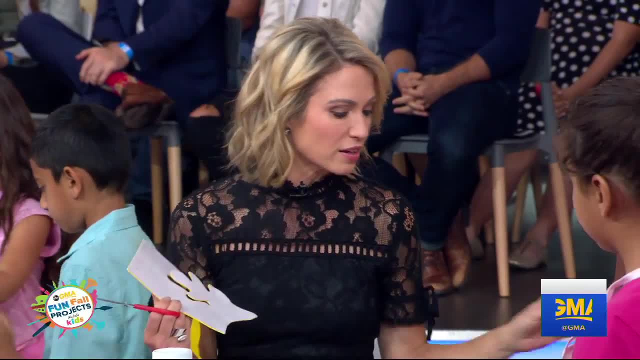 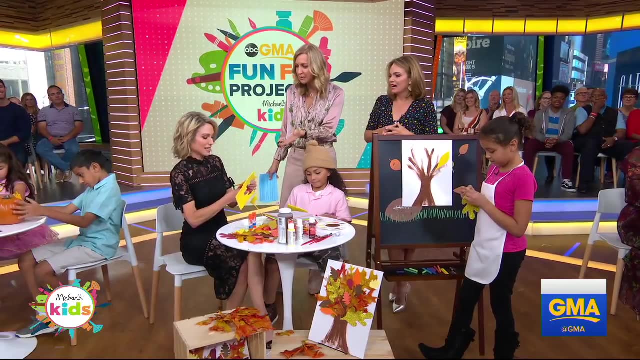 You can draw your own leaves and have all the different kinds you want. It's a little time consuming, right? Yes, Amy, you have that great country house: Grab real leaves as they fall and use the glue. Send the kids out and go and do that. 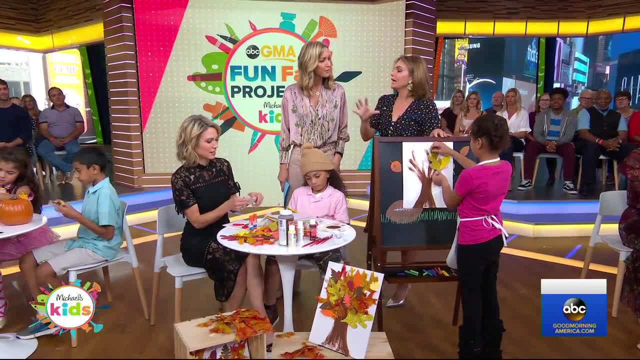 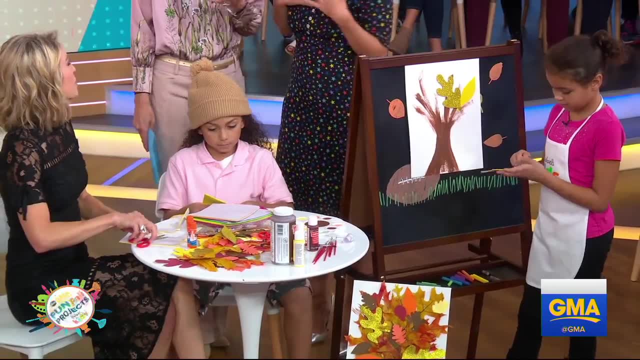 Use all the stuff- Really fun idea. It's so great. Also, at the end you can take this and frame it and put it in your house, So you have a fall piece of art project Piece of art. I love that. 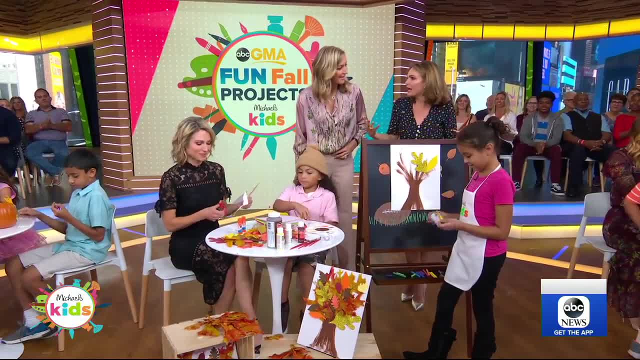 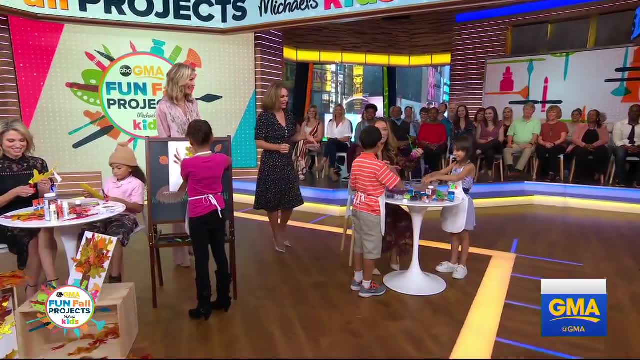 And I would love getting that as a parent Right. Anything homemade, I love getting it. Speaking of parents who like to behave like kids: my girl Ginger Z, I know Here she is. She's making slime already. I'm so impressed. 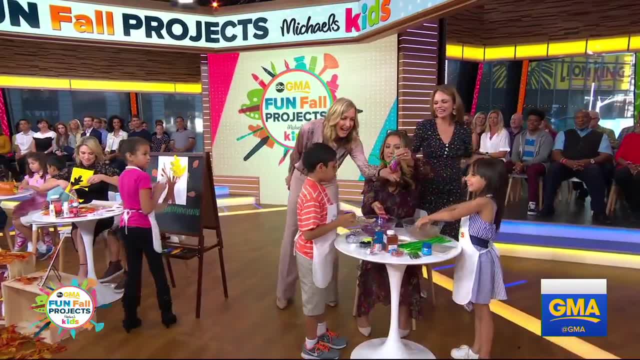 She just took the station. Can I show what Ginger's made? This is our slime guy. This is all about little scientists in the making with using, obviously, something we love- slime. Look, Slime, Slime. I have an 8-year-old. 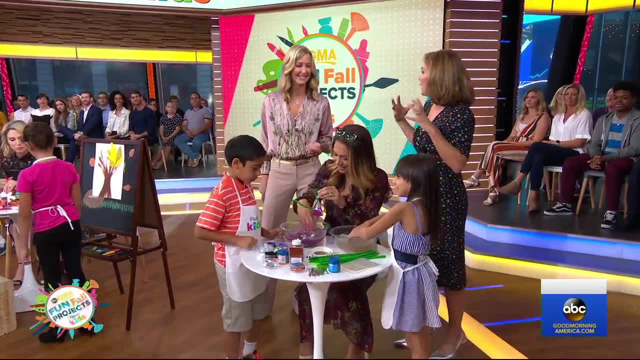 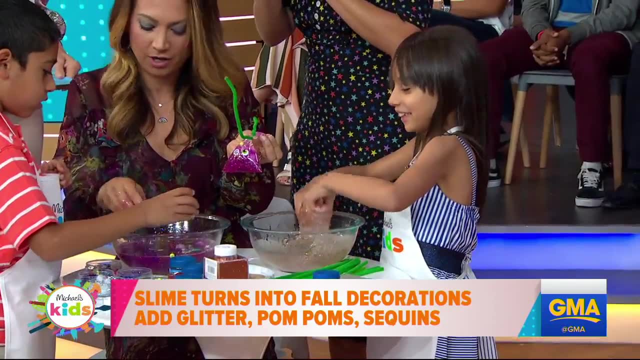